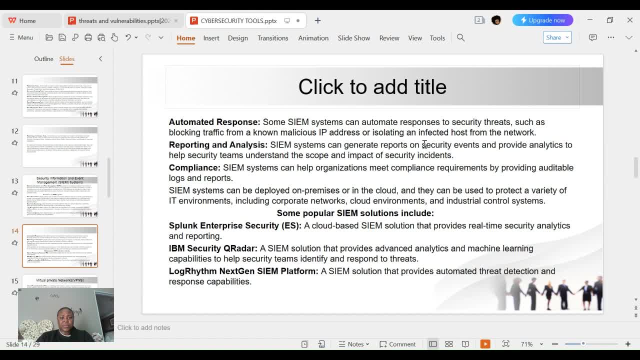 on known threats and vulnerabilities. Another one function is automated response. The SIEM system can automate responses to security threats, such as blocking traffic from a known malicious IP address or isolating an infected host from the network. Another one is reporting and analysis. The SIEM system can generate reports on security. 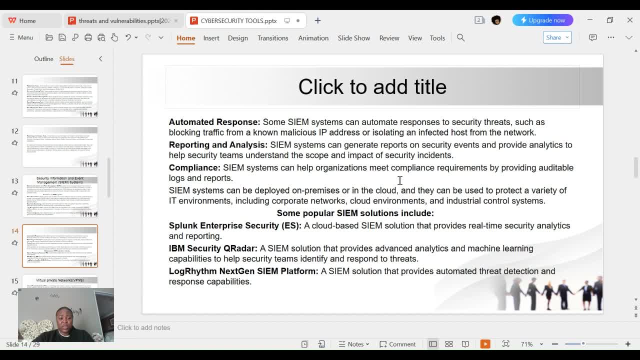 events and provide analysis to help security teams understand the scope and impact of security incidents. For compliance, the SIEM can help organizations meet compliance requirements by providing auditable logs and reports. SIEM systems can be deployed on premises or in the cloud, and they can 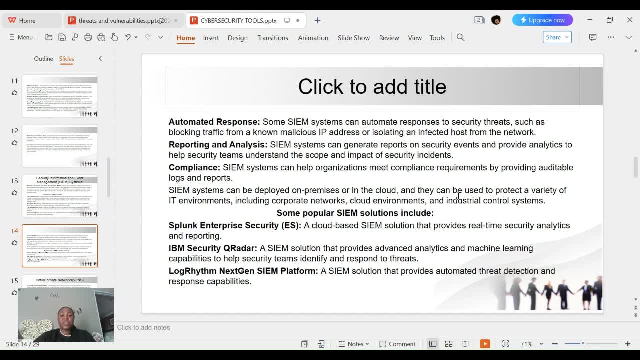 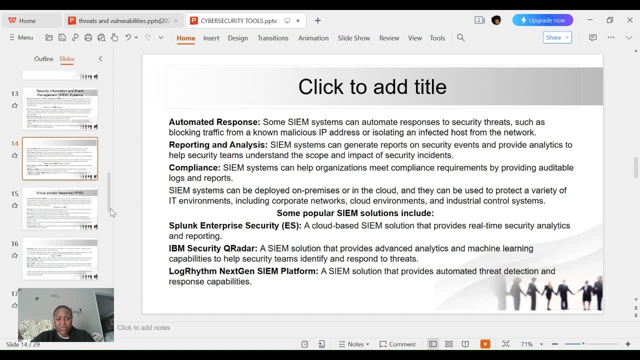 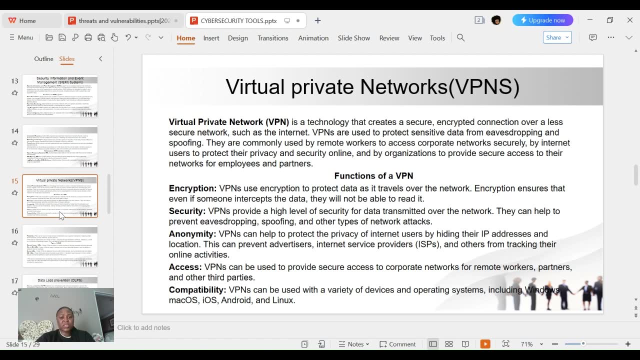 be used to protect a variety of IT environments, including compute network, cloud environment and industrial control systems. some of the examples of the same solutions are the splunk enterprise security, the ibm security radar and the long redeem next gen cm platform. another kind of cyber security tools is the 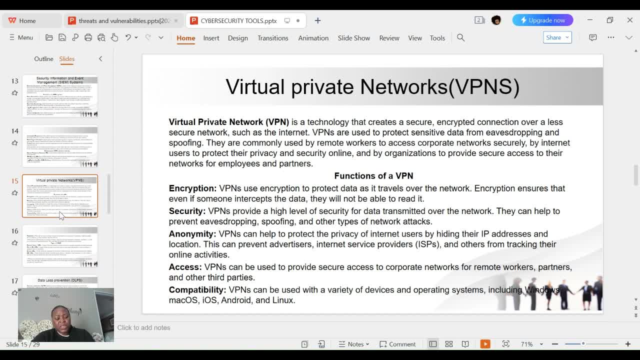 vpn. the vpns like traditionally. we know vpn as a system that can provide us a kind of an anonymity on the internet, but um, vpns also can be used to used as a cyber security tools. so the vpn is a technology that creates a secure, encrypted connection over a less secure network. 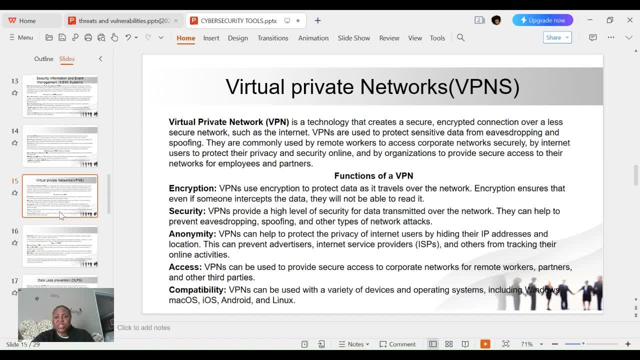 such as the internet. vpns are used to protect sensitive data from is dropping and spoofing. they are commonly used by remote workers to assess corporate networks securely, by internet users to protect their privacy and security online, and by organizations to provide secure access to their networks for employees and partners. what are the functions of? 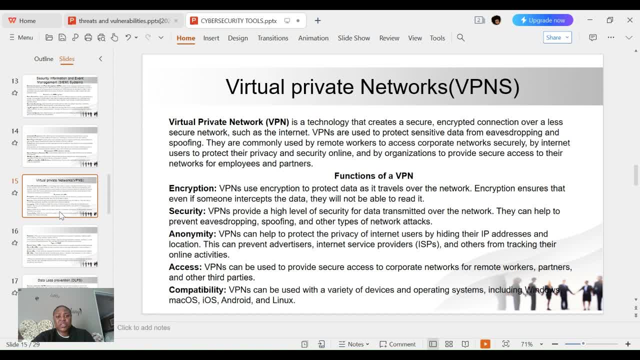 vpn for encryption. vpn vpns use encryption to protect data as it travels over the network. encryption ensures that even if someone intercepts the data, they will not be able to read it. so another function is for security. vpn provides a high level of security for data transmitted over the network. it can help to prevent is dropping, spoofing and other types. 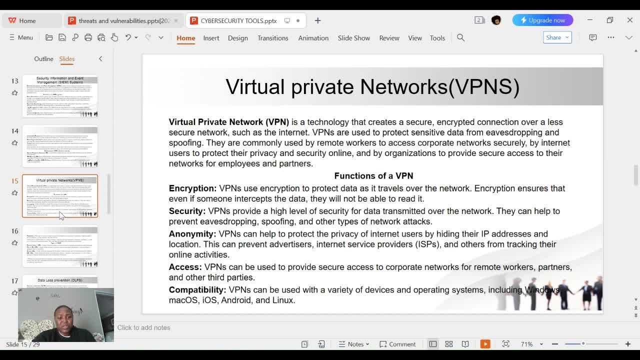 of network attacks. another function is for anonymity, which we all know. vpn can help to protect the privacy of internet users by hiding their ip addresses and location. this can prevent advertisers, internet service providers and others from tracking their online activities. vpns can be used to provide secure access to corporate networks for remote workers, partners and other tech parties. 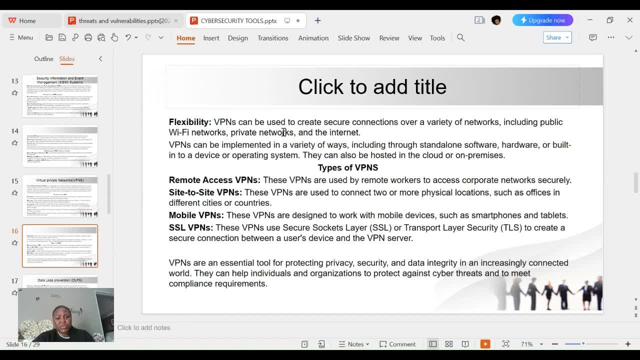 another function is for computer compatibility. vpn can be used with a variety of devices and operating system, including windows, mac os, ios, android and linux. another function is for visibility. vpn can be used to create secure connections over a variety of networks, including wi-fi networks, private networks and the internet. vpn can be implemented in a variety of ways. 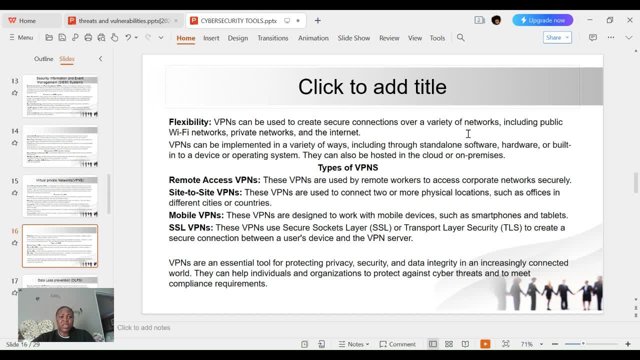 including through standalone software, hardware or built in to a device or operating device system. they can also be hosted in the cloud or on promises. what are the types of vpns? we have the remote access vpn. we have site to site vpn. we have mobile vpns and ssl vpns. i'll provide the 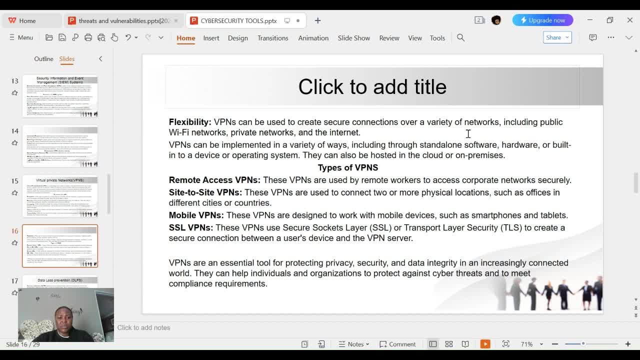 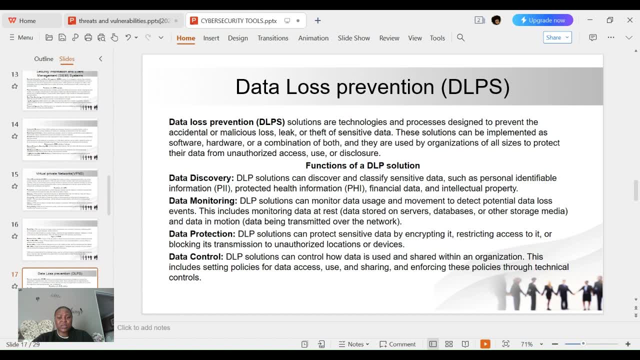 slide um in the google classroom so that you can read through it. vpns are an essential tool for protecting privacy, security and data integrity in an increasingly connected world. this can help individuals, organizations, protect against cyber threats and meet compliance requirement. another type of um cybersecurity tools is the data loss prevention solutions that are operational solutions. 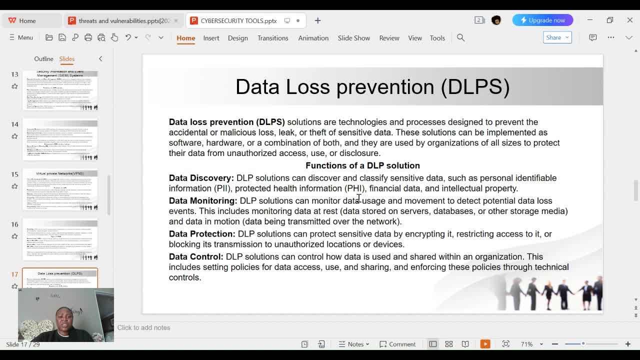 are technologies and processes designed to prevent the accidental or malicious loss, leak or theft of sensitive data. these solutions can be implemented as data, as software, hardware or a combination of both. they are used by organizations of all sizes to protect their data from unauthorized assets, use or disclosures. functions of dlp solutions that are discovering. 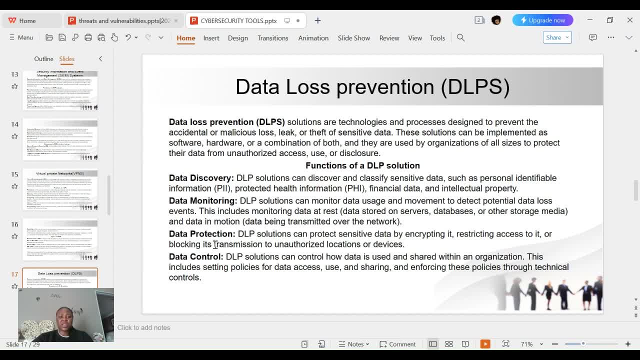 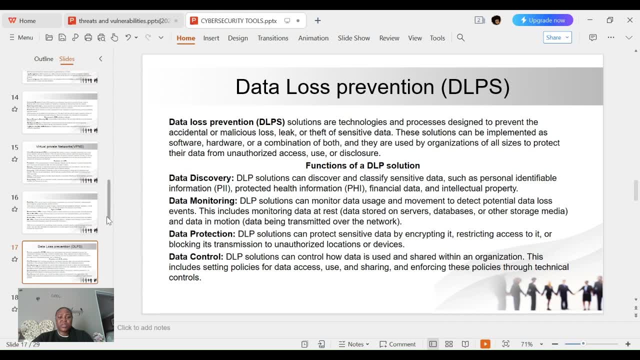 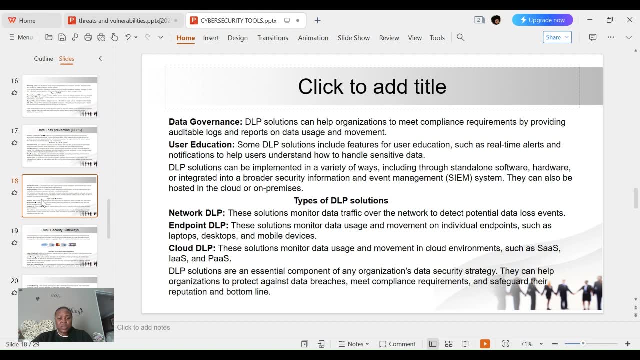 the observations can discover and classify sensitive data, such as personal identity, variables information, protected information, financial data and 宮s Interfacespecialtydlp solutions monitor their data and protect each data, and then also data control from our data controlкий тотlo, SRDB Djilboj and Data Confinement. 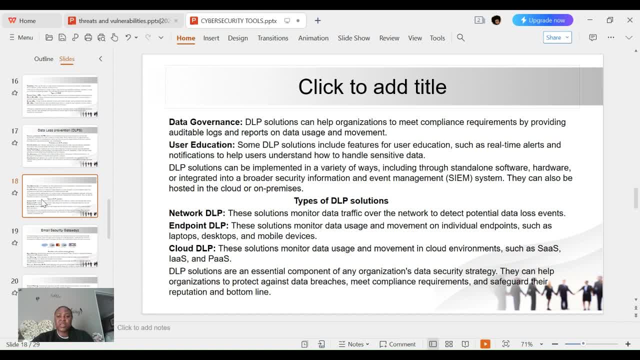 meric. DLP solutions can help organizations to meet climate compliance requirements by providing auditable logs and reports on data usage and movement and user education. DLP solutions include features for user education, such as real-time alerts and notifications to help users understand how to handle sensitive letters. DLP solutions can 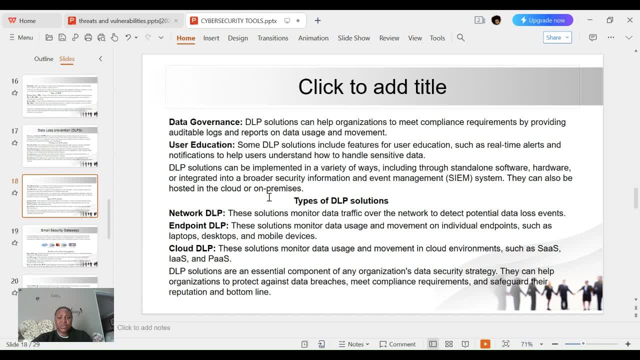 be implemented in a variety of ways, including through standalone software, hardware, or integrated into a broader solution- information and event management as the same which we talked about earlier. They can also be hosted in the cloud or on-premises. What are the types of DLP solutions? 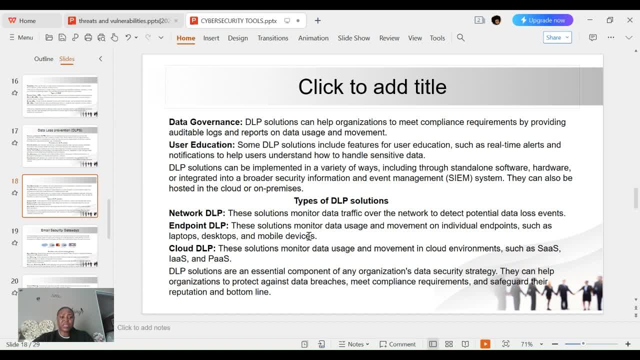 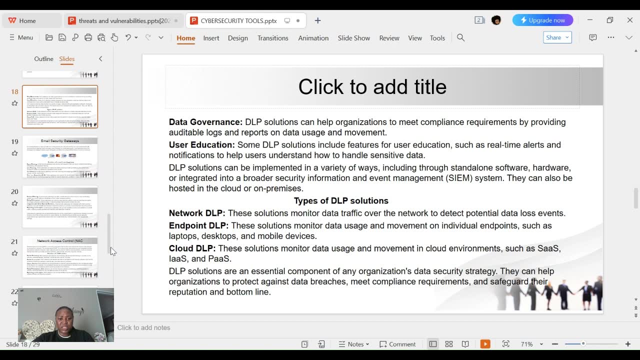 we have The network DLP, the endpoint DLP, cloud-based DLP. The examples of the cloud-based DLP are software as a service, login as a service and password as a service- sorry, platform as a service. DLP solutions are an essential component of any organization, Organizations data security. 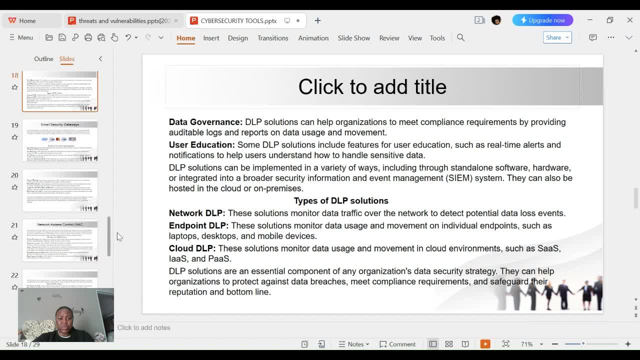 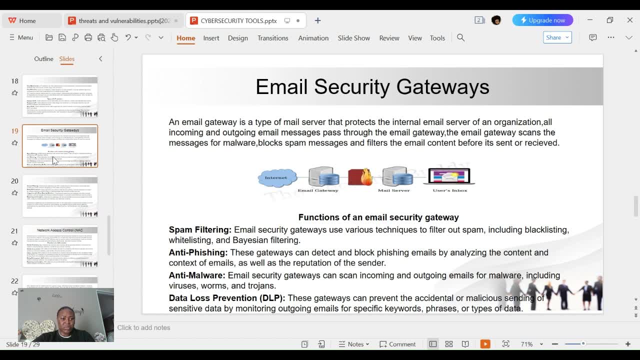 strategies. they can help organizations protect against data breaches, meet compliance requirements and safeguard their reputation and bottom line. So the next one is email security gateway. That's the next type of server security tools. The email gateway field has every information coming into your inbox. Email gateway is a type. 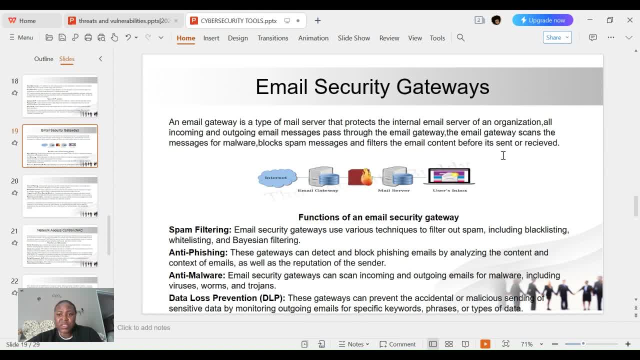 of mail server that protects the internal email server of an organization or incoming and outgoing email messages passed through the email gateway. The email gateway scans the messages from the mail way, blocks them and filters the email content before it's sent or received. Functions of the. 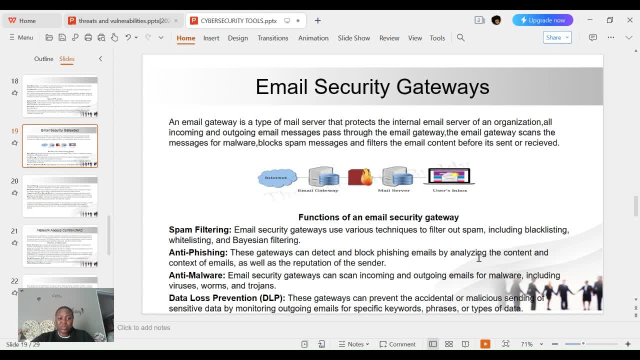 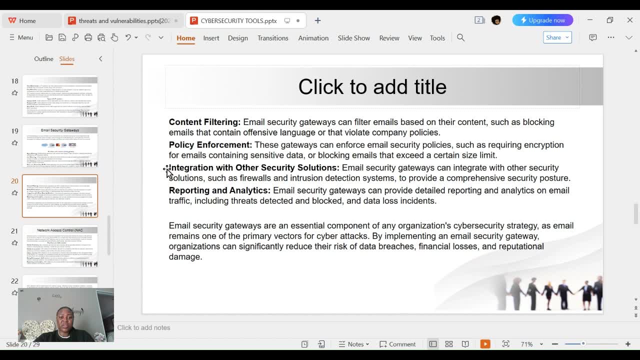 security. email security gateway is: filters spam. it acts on anti-phishing. it blocks phishing emails, content and context of emails, as well as the reputation of the sender. It is an anti-mailware. it prevents data loss and also it filters the content and policy. 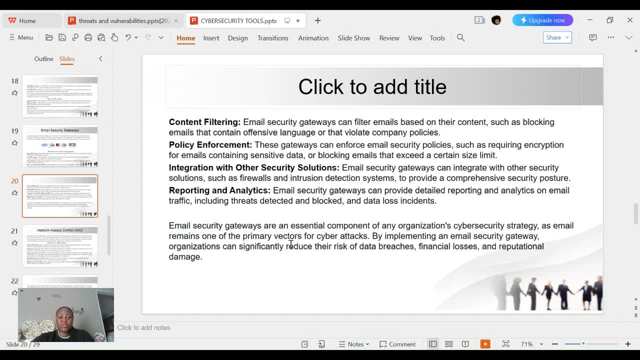 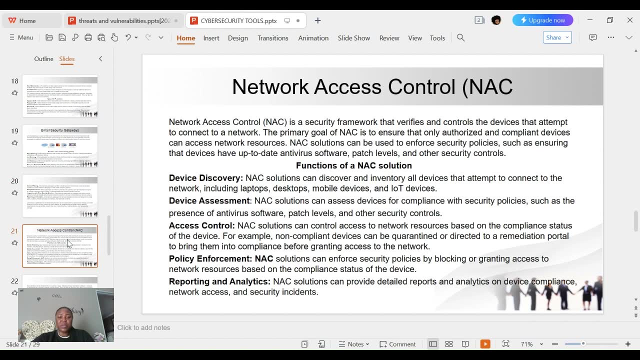 enforcement, integration with other security solutions, reporting and analytics. Email gateways are an essential component of an organization Cybersecurity trust strategy, as email remains one of the primary vectors for cyberattacks. By implementing an email security gateway organization can significantly reduce the risk of data breaches, financial loss and reputational damage. 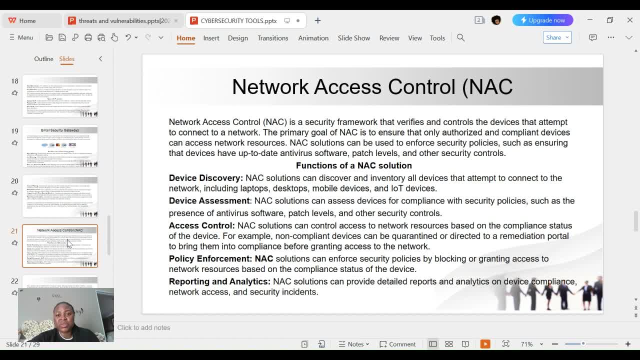 The next one is network access control. that is another type of cybersecurity tool. This is a security framework that verifies and controls the devices that attempts to connect to a network. The primary goal of NARC is to ensure that only authorized, compliant devices can access network resources. 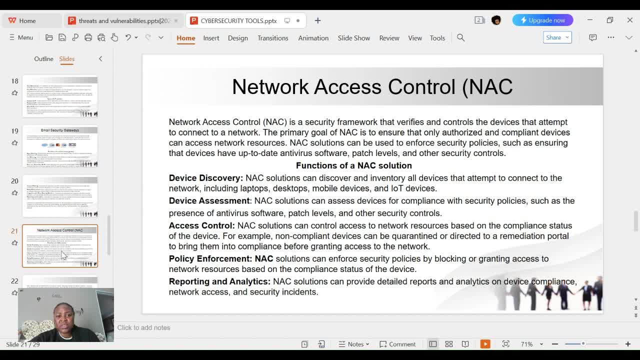 NARC solutions can be used to enforce security policies, such as ensuring that devices have up-to-date antivirus software patch levels and other security controls. What are the functions of NARC solution? Device discovery: NARC solution can discover and inventory all devices that attempts to connect to the network. 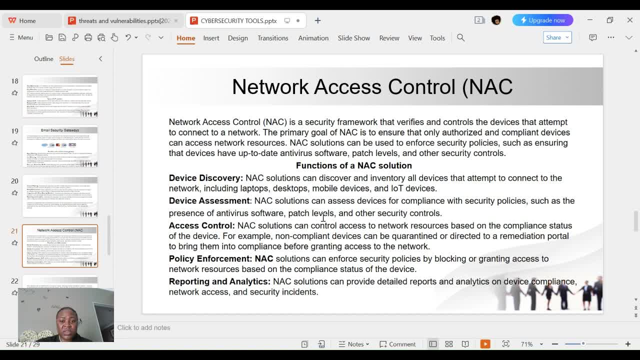 including laptops, desktop mobile devices and other devices. NARC solution can access devices for compliance with security policies, such as the presence of antivirus software, patch levels and other security controls. NARC solution can control access to network resources based on the compliance status of. 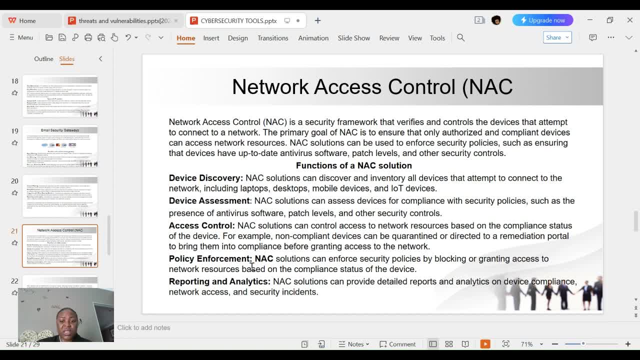 the device. For example, non-compliance devices can be quarantined or directed to a remediation portal to bring them into compliance. For example, non-compliance devices can be quarantined or directed to a remediation portal. For example, non-compliance devices can be quarantined or directed to a remediation portal. 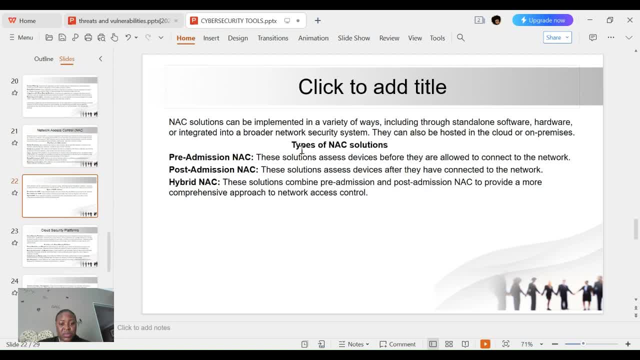 NARC solution canully address objectsipperig door. NARC solution can operate on a high degree違造 с destructible device without banning from Черimoranked NARC tool, while the device is not power off at all. 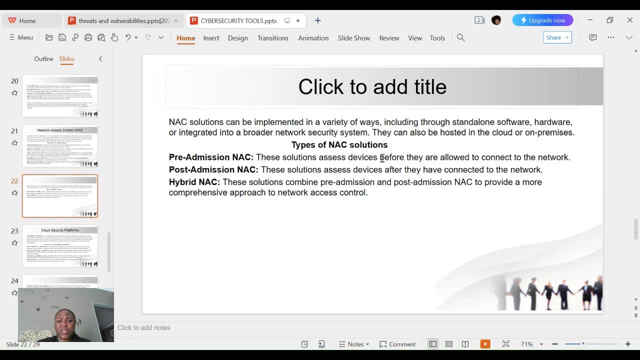 NARC solution can be implemented by a variety of ways, including through standalone software and hardware, or integrated into an established network security system. NARC solution can be implemented by a variety of ways, including through standalone software and hardware, or integrated into an established network security system. 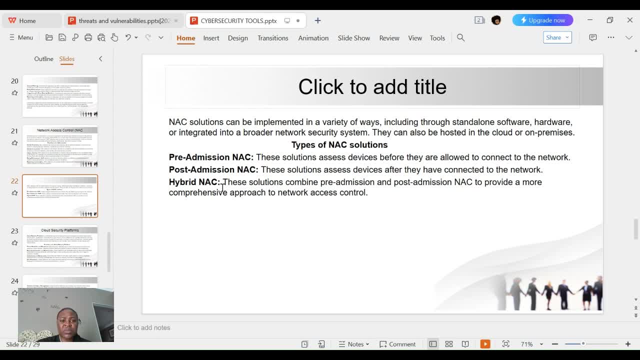 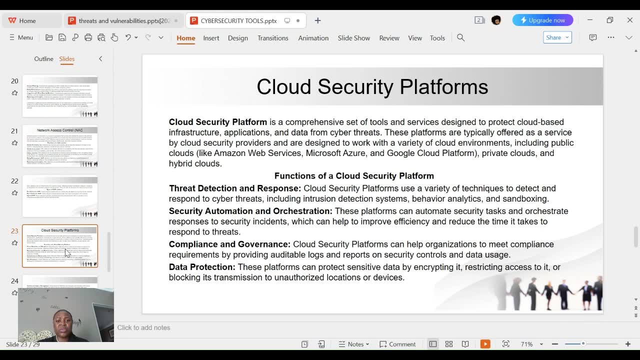 NARC solution can apply by is table, desktop and operating system using two devices. So Types of NARC solutions: we have pre-admission NARC, we have post-admission NARC, we have the hybrid. It's a solution which combines the pre-admission and the post-admission NARC to provide a more. 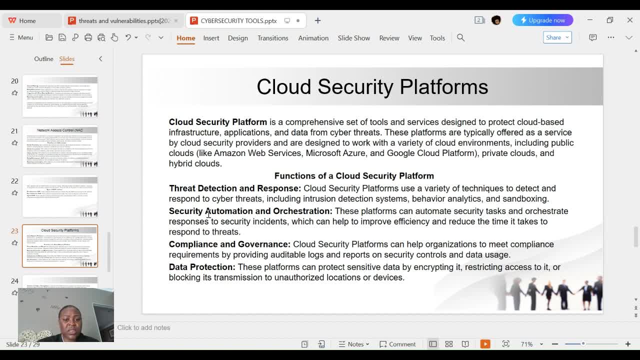 comprehensive approach to network and access control. Another type of cybersecurity tool is the cloud security platform. The cloud security platform is a comprehensive set of tools and services designed to protect cloud-based infrastructures, applications and data from cyber threats. These platforms are typically offered as a service by cloud security providers and also. 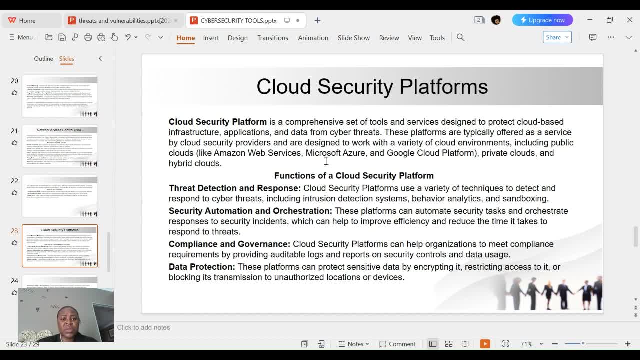 designed to work with a variety of cloud environments, including public clouds. Examples of these providers are like the Amazon Web Service, the Microsoft Azure and the Google Cloud Platform, which are the three most popular ones, private clouds and hybrid clouds. Examples of a cloud security platform entails threat detection and responses. 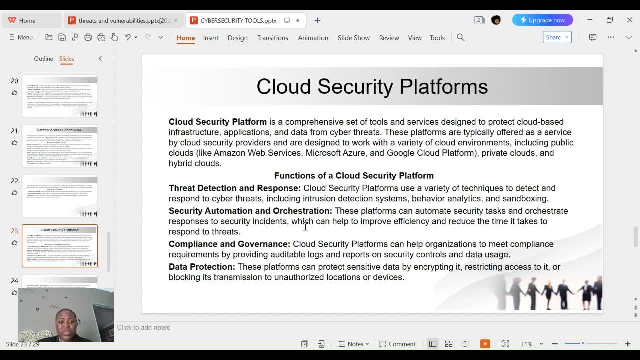 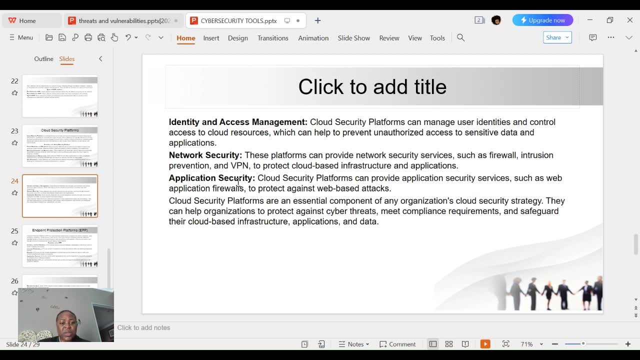 Cloud security platforms use a variety of techniques to detect and respond to cyber threats, including intrusion detection systems, behavior analysis, sandboxing. Another function is for security, automation and orchestration. Another function is compliance and governance. Another function is for data protection. 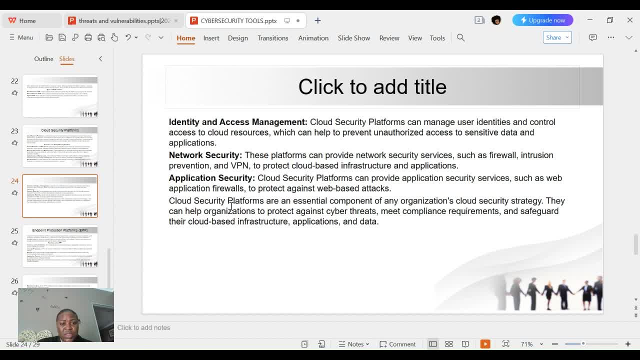 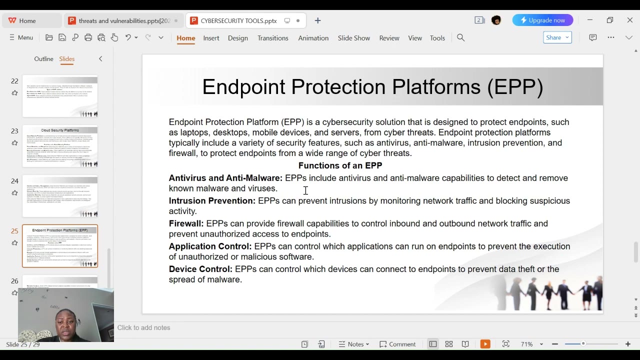 Thank you. Another one is for identity and access management, network security and application security. I can't leave it through. the slide will be on our Google Classroom. So cloud security platforms are an essential component of any organization's cloud security strategy. They can help organizations protect against cyber threats with compliance requirements. 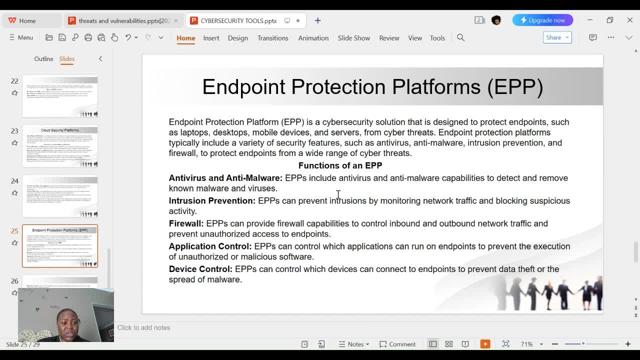 and safeguard their cloud-based infrastructure, applications and data. Another type of cybersecurity tool is the Endpoint Protection Platform. Endpoint Protection Platform is a cybersecurity solution that is designed to protect endpoints such as laptops, desktops, mobile devices and servers from cyber threats. 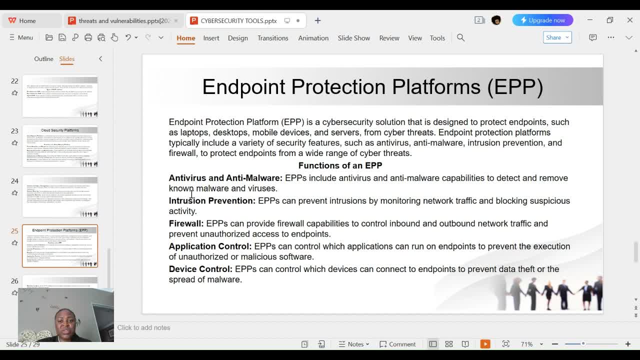 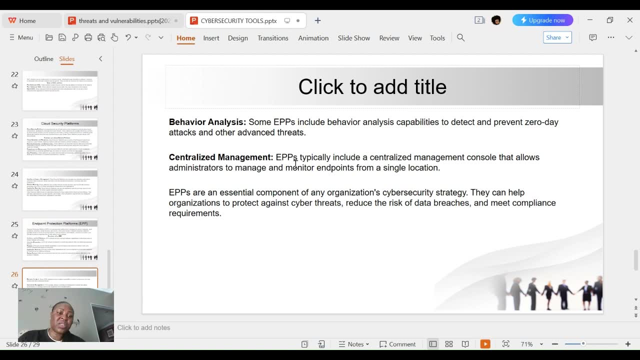 Endpoint protection platforms typically include a variety of security features, such as antivirus and anti-malware, intrusion prevention and firewall, to protect endpoints from a wide range of cyber threats. Functions of an EPP is an antivirus and anti-malware. it acts as an antivirus and anti-malware intrusion. 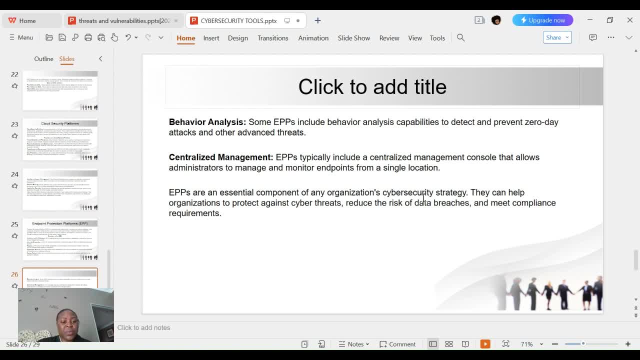 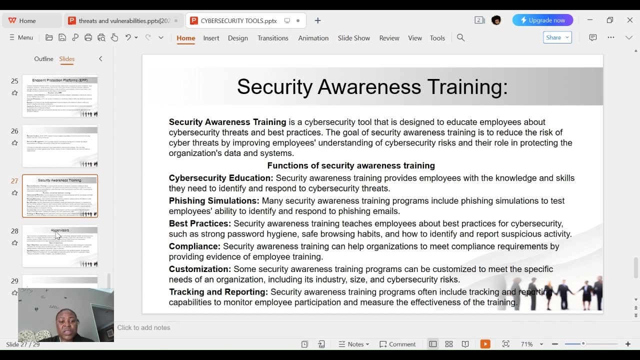 prevention, firewall application control, device control, behavior analysis, centralized management- EPP- is an essential component of an organization's cybersecurity strategy. It can help organizations to protect against cyber threats, reduce the risk of data breaches and meet compliance. It can help organizations to protect against cyber threats, reduce the risk of data breaches. 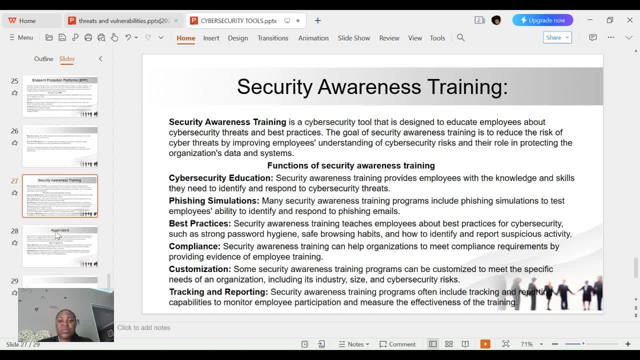 and meet compliance. The last but not the least is Security Awareness Training. So the Security Awareness Training is a cybersecurity tool that is designed to educate employees about cybersecurity threats and best practices. The goal of cybersecurity awareness training is to reduce the risk of cyber threats by 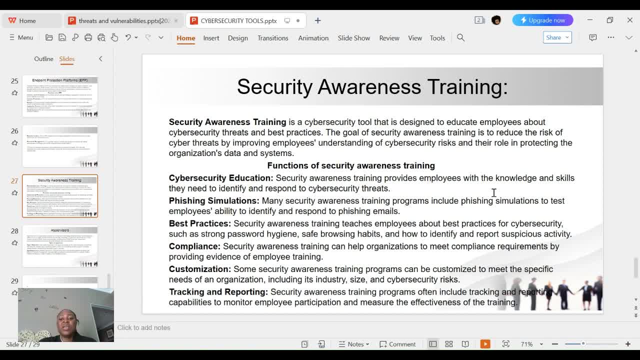 improving employees' understanding of cybersecurity risks and their roles in protecting the organization's data and systems. Part two functions of security awareness training is cybersecurity training. security awareness training provides employee with knowledge and skills they need to identify and respond to cybersecurity threats, phishing simulations, many. 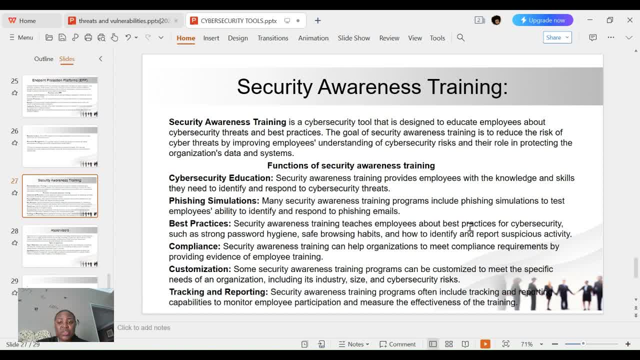 security awareness training programs include phishing simulation to test employees ability to identify and respond to phishing emails. best practices: security awareness training teaches employees about best practices for cyber security, such as strong password hygiene, safe browsing habits and how to identify and report suspicious activities. another functions of security awareness training is compliance security awareness training. 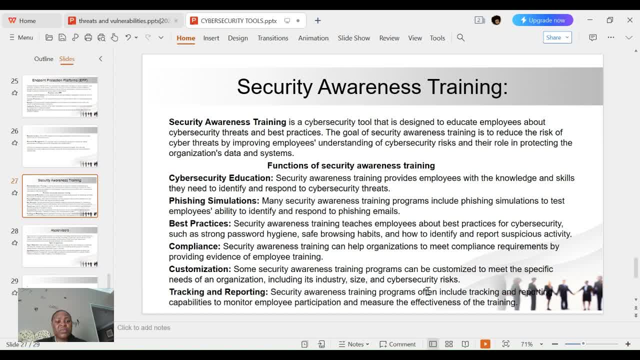 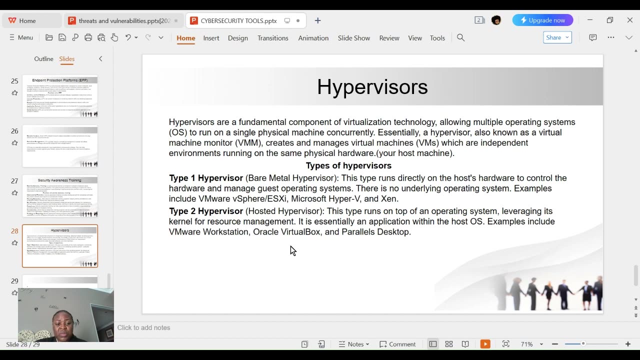 can help organizations to meet compliance requirement by providing evidence of employee training. another one is customization. some security awareness training programs can be customized to meet the specific needs of an organization, including its industry size and cybersecurity ethics. another function is for tracking and reporting. security awareness training programs often include tracking and reporting capabilities to monitor. 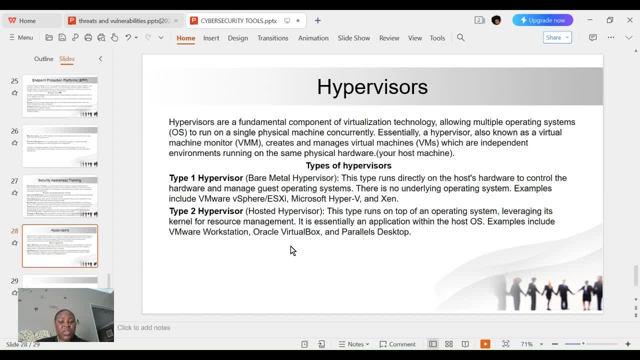 employees participation and monitor the effectiveness of the training. so the last topic we're going to talk about today is the hypervisors, because we'll be installing our tools tomorrow. that will be handled by Mr Boniface. hypervisors are a fundamental component. okay, what are hypervectors? sorry, hypervectors are a fundamental